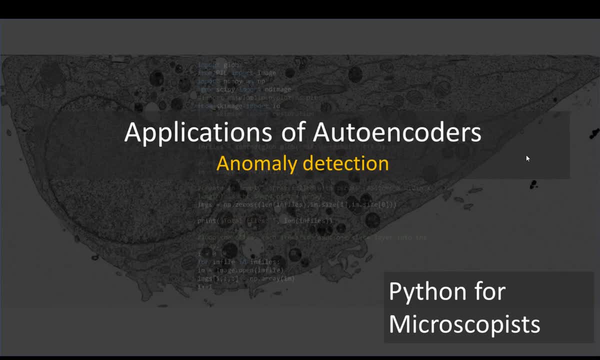 technique. In fact, instead of working on images, I actually created synthetic data in Python, So let's use the same technique. In fact, instead of working on images, I actually created synthetic data in Python, So let's use the same technique, In fact, instead of. 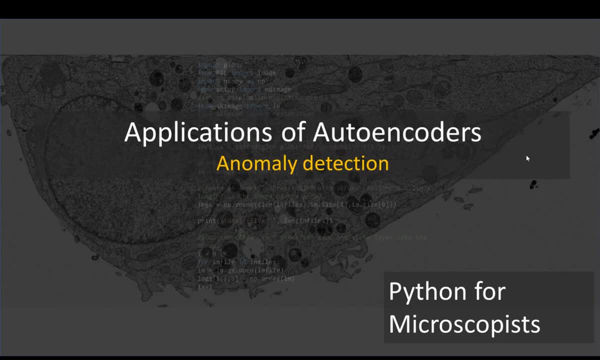 a Excel or a CSV file where I have two columns and introduced some anomalies occasionally so we can read that data. But again, as long as you can get your images into a form that you can use in your deep learning or autoencoders, then you can use any data because for a computer 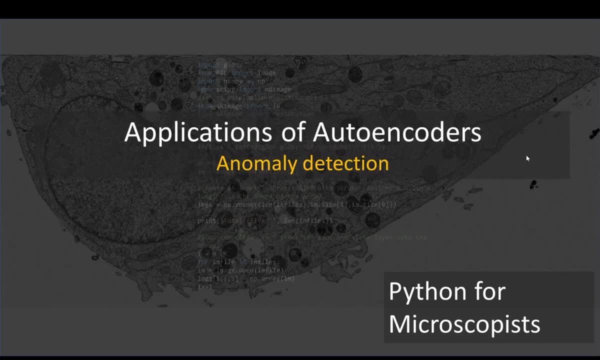 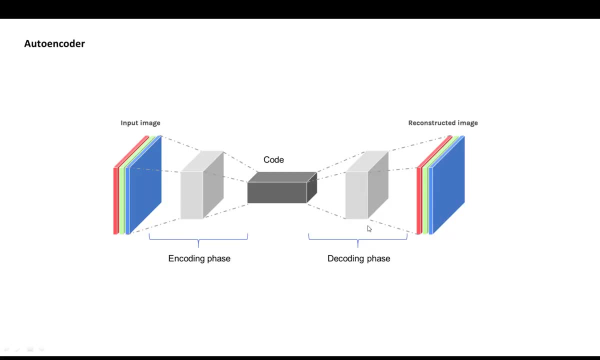 it doesn't care if it's an image, if it's a sound file or if it is a video file or any other type of data. So with that understanding again, let's also look at, remind ourselves, what autoencoders are. Again, it's basically neural networks that are organized such a way that the input image, the dimensions, are reduced, and then, which is called encoding phase, and the dimensions are again brought back or upscaled to the original size. and this is the decoding phase. 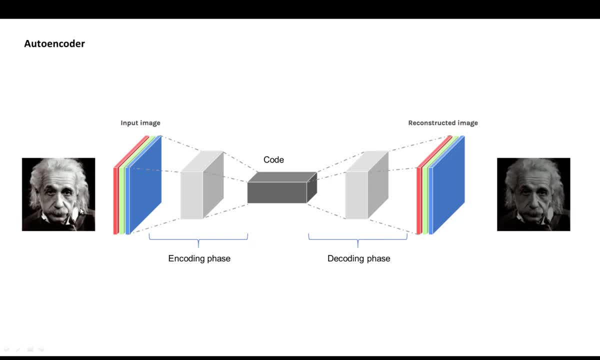 And the idea of autoencoder is to reconstruct the original image by going through this process, and during this process of reconstruction, the weights and biases are adjusted, meaning you're creating a model that you can use to reconstruct future images. So we take advantage of this concept by feeding the input you know, for example, for denoising, we just supplied a noisy image and reconstructed a healthy image, meaning during the training phase, 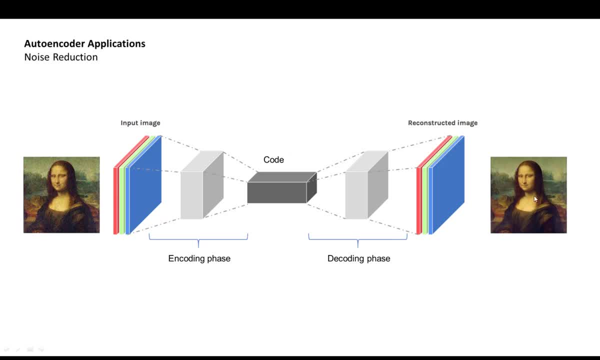 you know, you know, you know, X is going to be the noisy image and our Y, when we are fitting a model, is going to be the healthy image. Now for let me skip. actually we are looking at anomalies, so let's actually look at this anomaly detection example here. 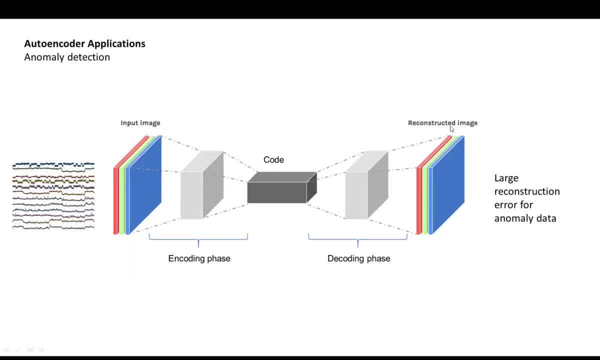 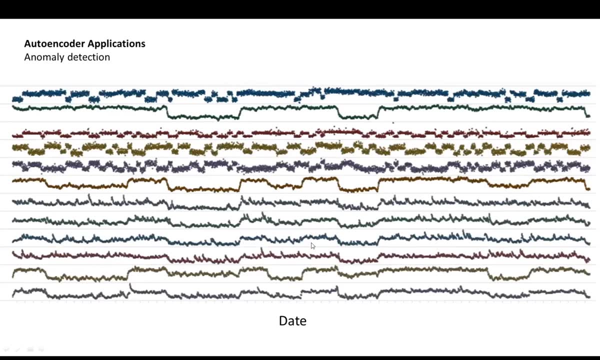 So you have a whole bunch of data, and now what if we- I should mention you have a whole bunch of annotated data. right, Everyone has data. Not many people have the luxury of annotated data, which means someone probably told that. okay, wherever you see these kind of spikes. 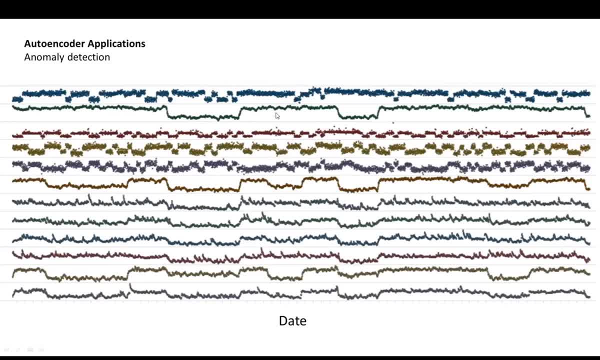 this is not good. this is bad response. Wherever you see something else, that's good. Maybe the spikes are expected, but as an expert, you need to say that. okay, you need to label this data by saying: okay for this stream of data which could be the power output of one of the lasers in your confocal microscope. okay, 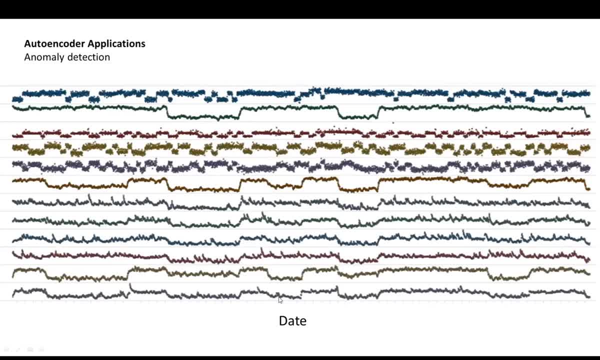 So, okay, that looks very stable and you may set some threshold and say, okay, this is an anomaly, this is an anomaly. tell me when that happens. right, And this could be, I don't know. the detector sensitivity. 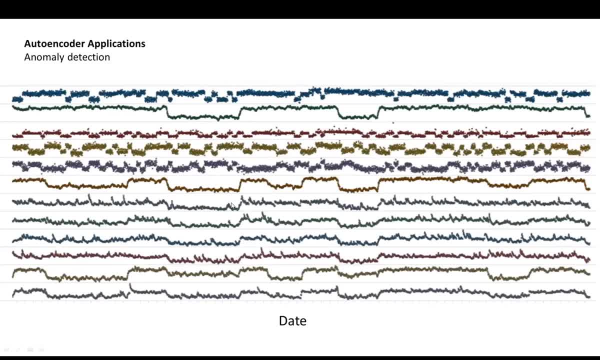 Yeah, and this could be something else. So you may be working with a whole bunch of streams of data coming from one single microscope or any other example you can think of. If you work on some other instrument you know, or some other situation, you'll have a whole bunch of data. 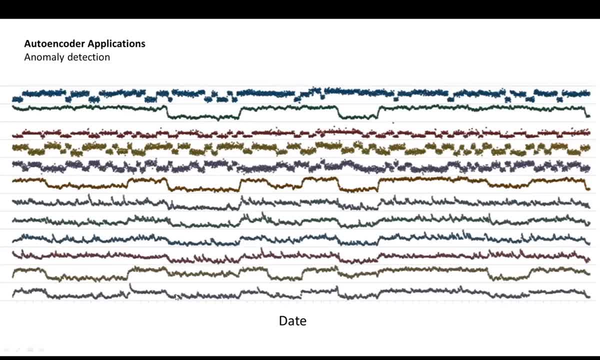 Well, this can be even sports data: This can be how my quarterback is performing and this is how my running back is performing, and per game, and you can actually have like a date versus the performance and then you can say, okay, what's an anomaly. 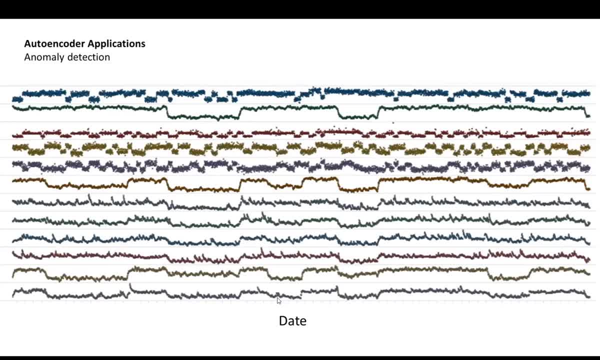 Is my quarterback distracted? I don't know. you know, is the quarterback healthy or not healthy? So you can think of many situations. you know where you can use this anomaly, What is normal and what is abnormal, right, So how do we detect anomalies? 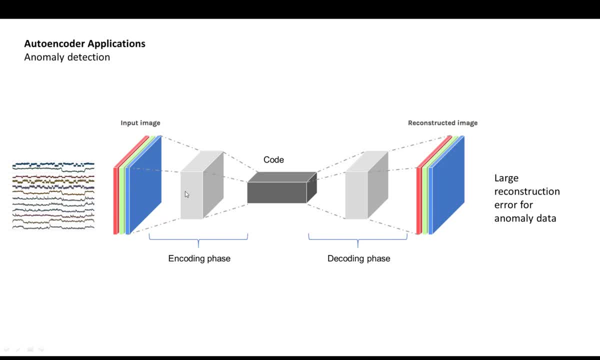 It's very simple. You just train the system on a whole bunch of good data, meaning non-anomaly data, right? And then anything that falls out of that norm is automatically labeled anomaly. okay, That's very simple, That's it. 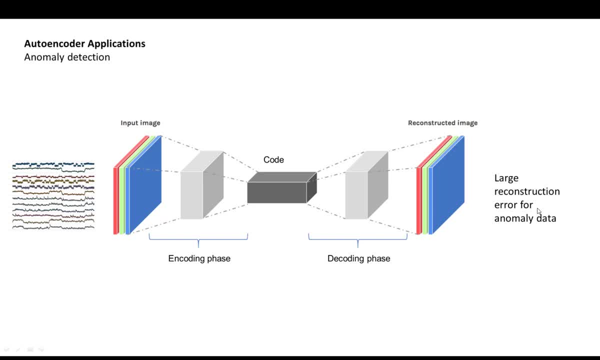 So, which means we are looking at the reconstruction error for our anomaly data. For regular data, the reconstruction error would be lower compared to the reconstruction error for the anomaly data. That's it. So we take this simple thing to actually build our auto-encoder for anomaly detection. 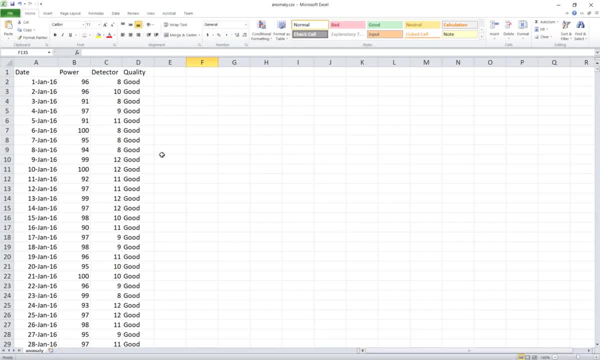 So let's go ahead and jump in And, by the way, the data I synthetically created is okay. there is a date. I'll start. I'm recording from January 2016.. It goes all the way to December 2019.. 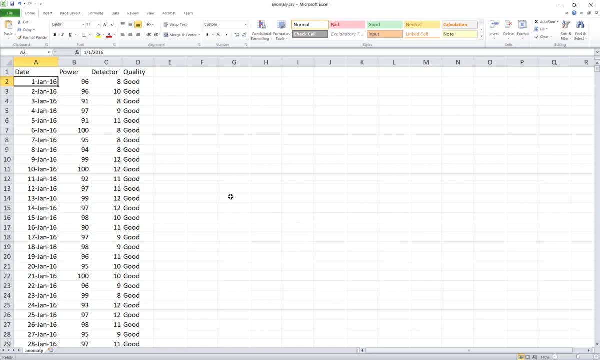 I'm recording this in January, early January of 2020.. So for about three years I have the data of you know, for the power of the laser, for example, and the detector sensitivity, And someone labeled it as good or bad, right. 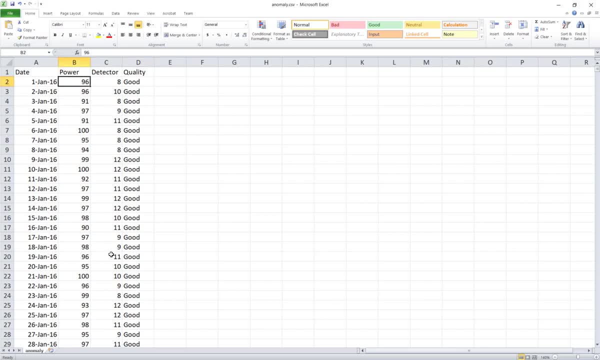 So if the power is centered around- I believe I did 95 or something- then it is good, And if the detector is centered around 8 or 9. It is good. Now, if it goes below a certain threshold, it is bad. 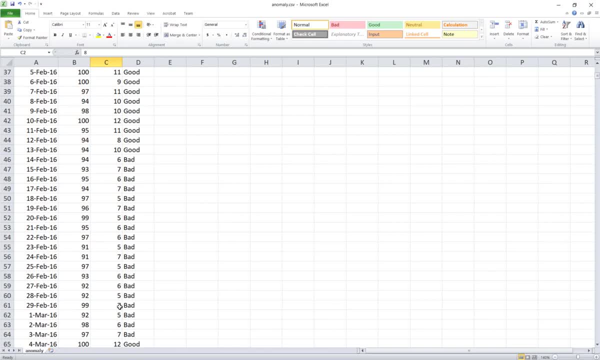 This is obviously a synthetic data, meaning you know I'm just using it for the tutorial purpose. But in real life situations can be a bit more complicated. In fact, you can basically say: bad is when you're- let's say you're- working with an X-ray source. 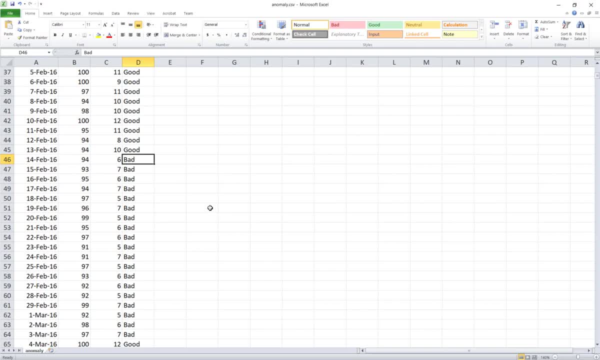 And your X-ray all of a sudden goes, you know, stops, right, So that's bad. So in real life you may have situations where you have real data, where things went bad, But for now, let's just look at this. 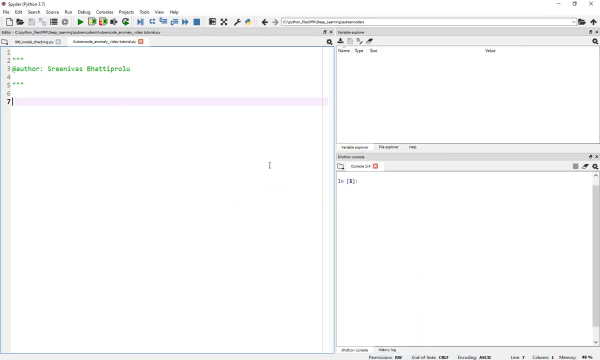 So this is in a CSV file. Again, I don't want to make this a pandas tutorial, because I've already done that in the past, So I will just go ahead and copy and paste the code, But I'll explain it while we are going along. 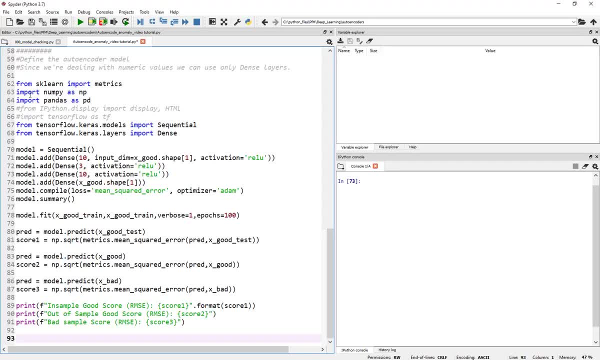 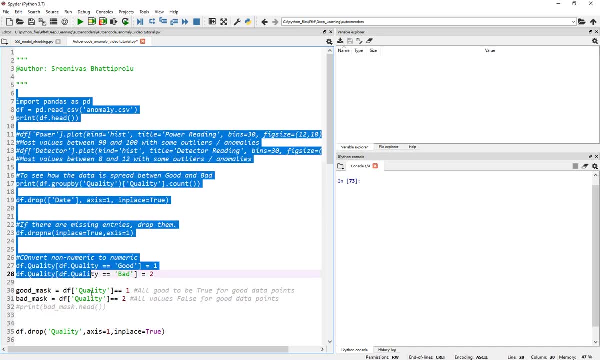 Okay, Okay, let me paste the code I copied from this other document. And there you go, And I'm not going to dwell too much time on how the data you know got structured, Although I think it makes sense to explain that. 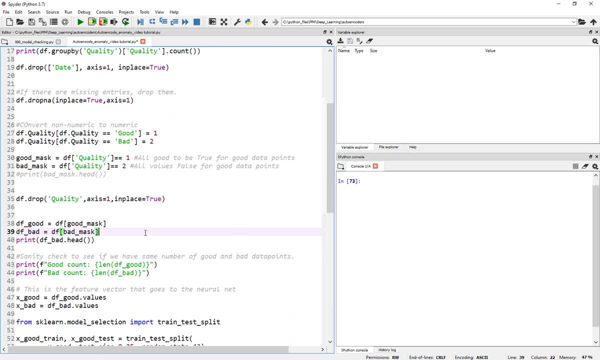 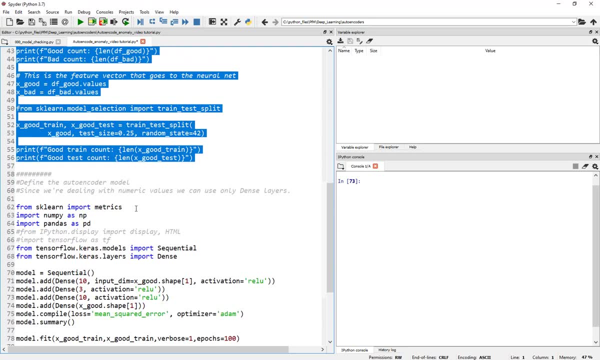 But again, at the end of this, what we are trying to do is all this part. Let me quickly mention all the up to here. like the first 40 lines is okay. how do I structure my data After that? it's very simple. 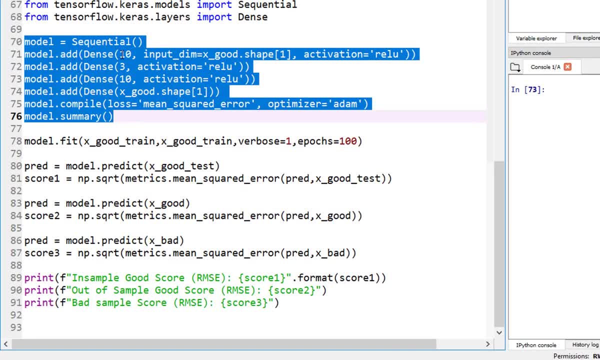 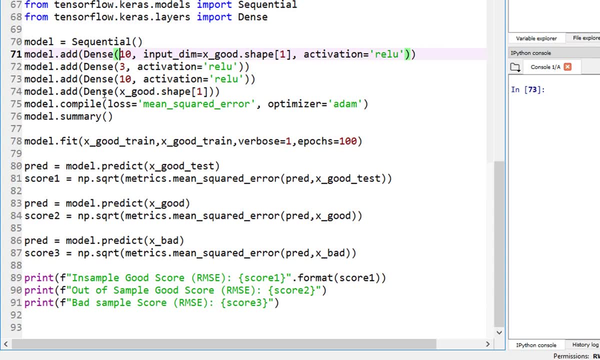 It's. basically. this is my model, sequential, starting with again. I'm only using dense layers here because this is a stream of data and not images. Okay, if it is images, then I recommend using the convolutional layers, because convolutional layers 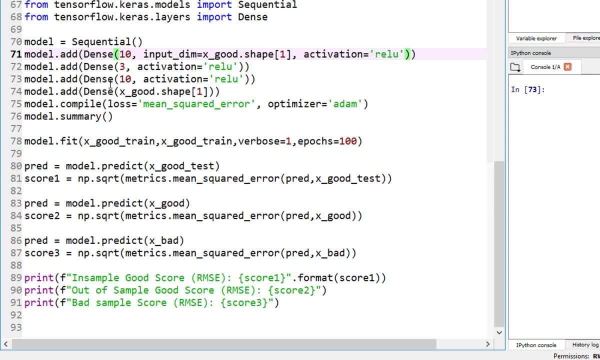 you work with these 2D images right, So the spatial information is retained and you can leverage the spatial information you know to gain insights into your data. Now, here for dense layers, you have to collapse your 2D into 1D vector. 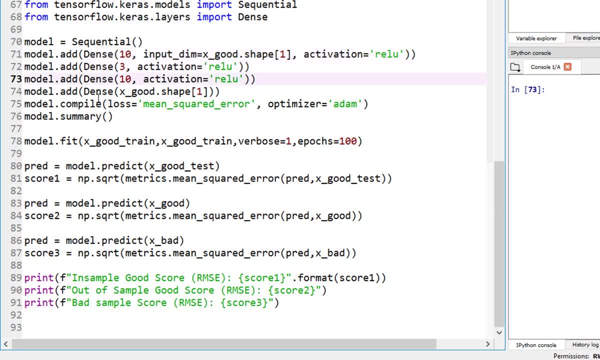 So, for images, I do not recommend working with dense layers unless you get to the classification point, which is not what we are discussing right now. We are discussing autoencoders. So again for stream, So for streams of data, dense layers are okay. 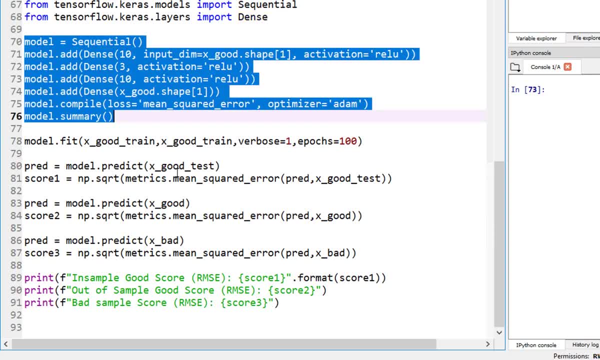 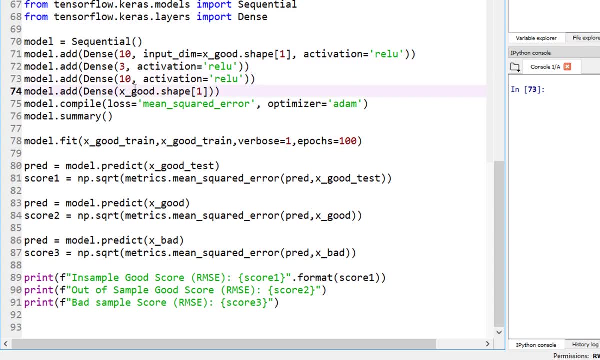 Okay, so this is this part is our autoencoder. that's it, okay. It starts with a dimension of 10,, goes down to a dimension of 3, and then reconstructs back to 10, and now, finally, we are reshaping it and printing it out. okay. 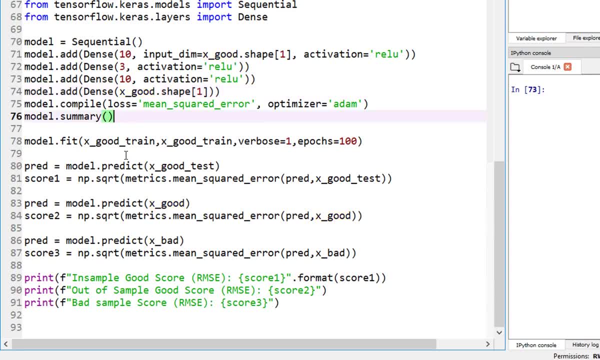 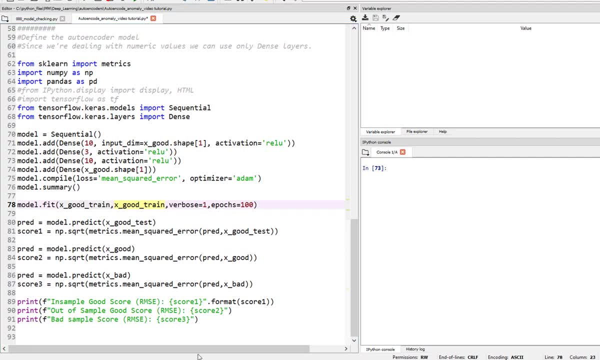 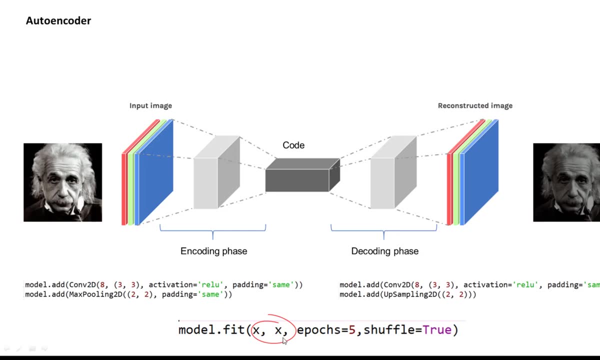 And at the end of this, we are going to fit this model to our- you know, to the same right. So again, let me go back to the presentation, The presentation I showed you earlier. eventually, we are fitting the model on X and X, meaning we are mapping X to X itself. 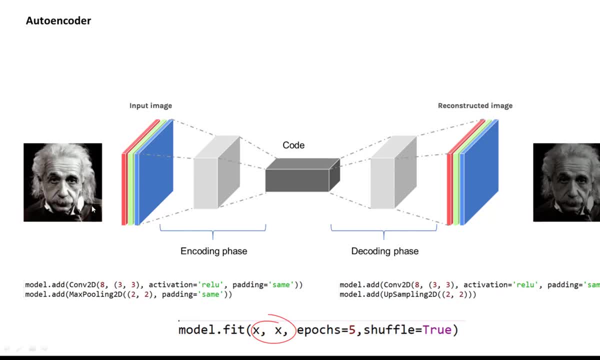 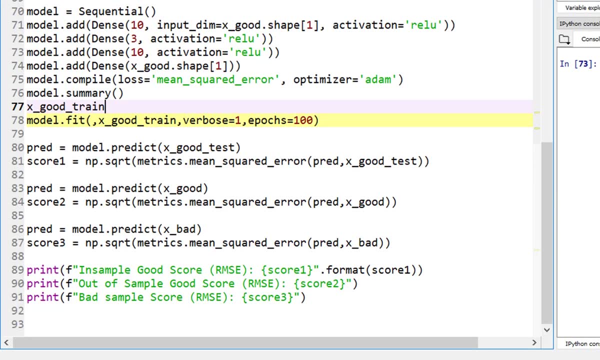 Our output is same as our input. This is what an autoencoder is. That's exactly what we are trying to do here. okay, I'm going to. I'm going to create a vector called X. sorry, I didn't mean to change it. 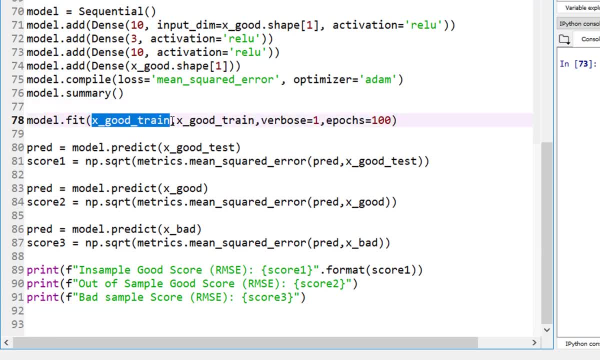 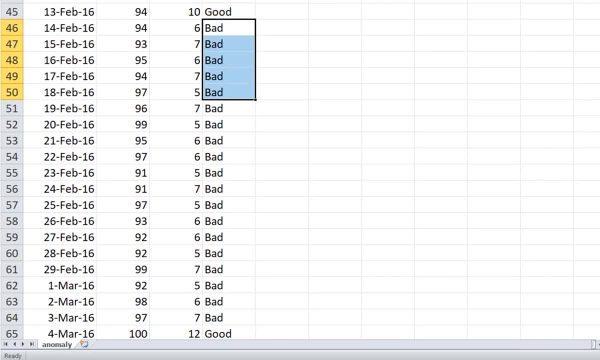 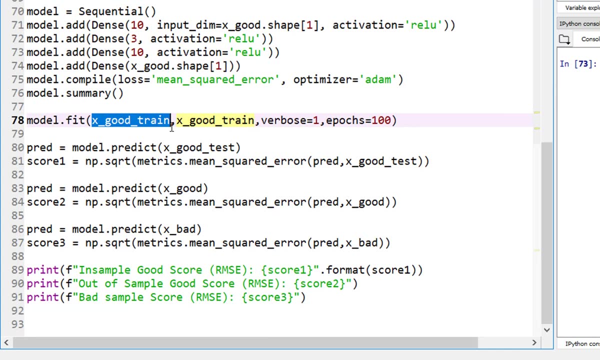 I'm going to create a vector called X underscore- good underscore train, obviously representing all the good data points that I showed you earlier, all the good data points. And for all the bad data points, or data points that are tagged as bad, I'm going to use that as my validation data for anomalies, right? 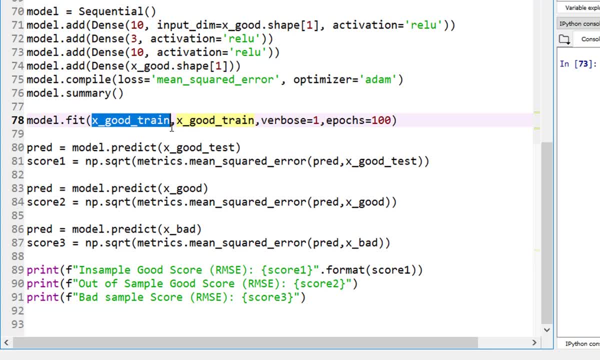 Good is not an anomaly, Bad is an anomaly. So the model is fit on the good data, both X and X. okay, Both are good, and let's do it for 100 epochs. and then I'm going to predict it on the X good test data set that we are holding out, you know, for testing, for validation. 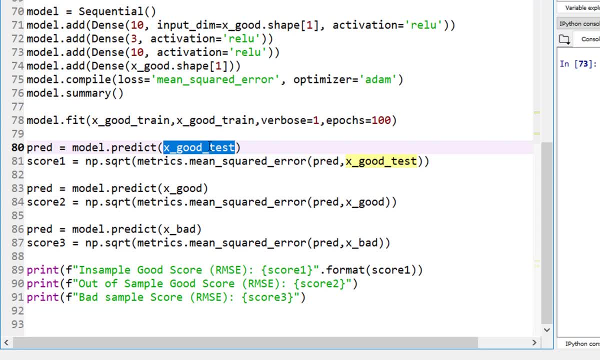 So the model is fit on the good data, both X and X. okay, Both are good, both are good. going to predict it on the mean squared error on the bad data set is my hope. again, what basically the by design? what it's going to do is anything that is good. the mean squared error should be. 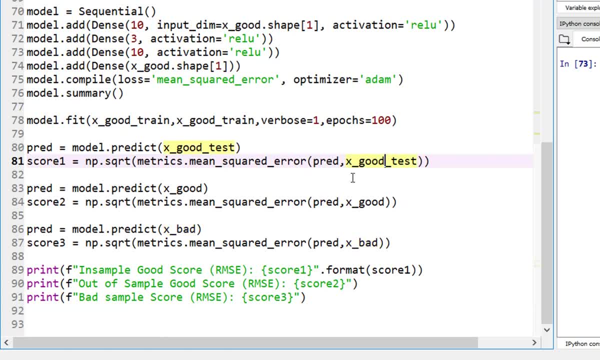 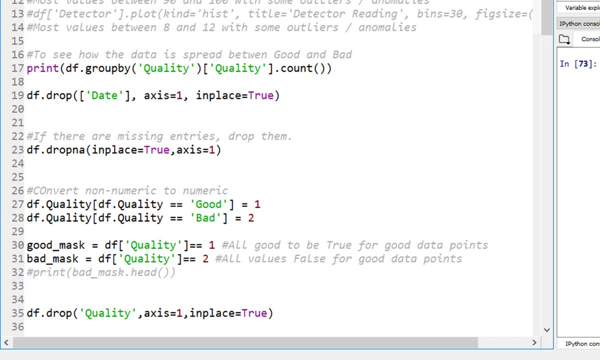 within certain acceptable limits. right, so that's the presumption, and anything that is a bad data set. the mean squared error should be larger compared to these two, and then we are going to print it out. okay, so this is how we design this, and just to give a quick overview of how I'm 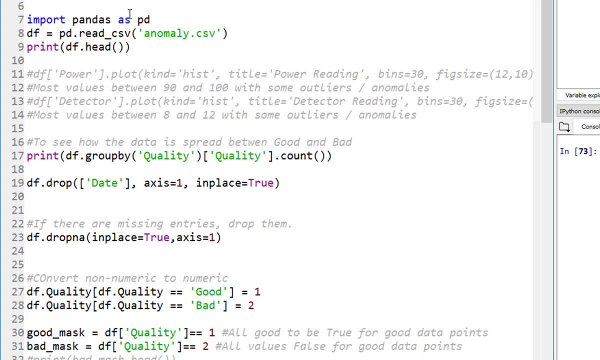 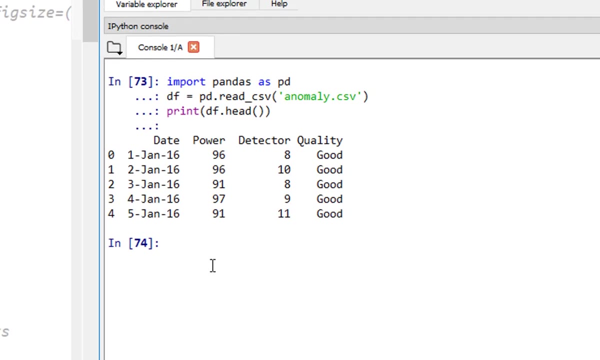 handling the data. again, I'm using pandas database- I mean, sorry, pandas library- to handle the data, and I did cover this topic in one of my previous tutorials, so please go ahead and watch it if you want to learn more about it. so step number one: importing our anomaly dot CSV file, and we 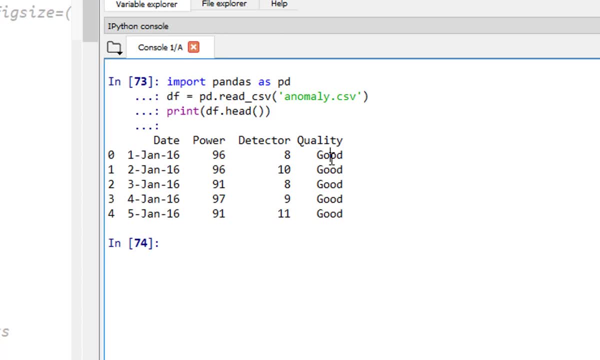 have four columns: date, power detector and quality. okay, now date is irrelevant for us because we're not doing any forecasting. we are just trying to build a model using the good data sets, and then anything that's not good is going to be a anomaly. okay, so this means we have to drop some data from from here. step number one: drop the date column. okay, 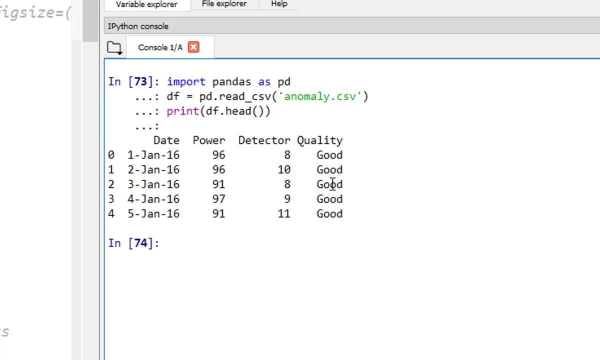 because that's irrelevant. step number two separate the good data points from the bad data points, because we want to train our model only on the good data points. so these steps are all designed to do exactly that and finally, of course, as we are doing this, we would like to 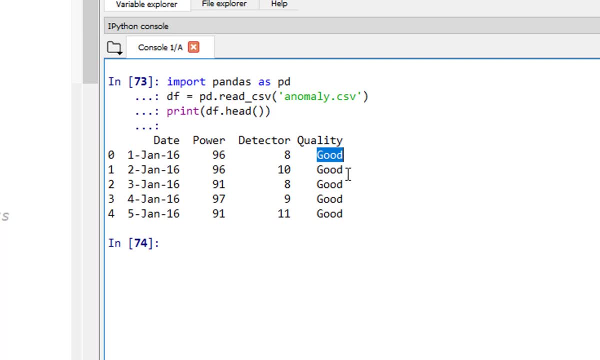 replace the text good with a value of one, text bad with a value of two, because obviously the, the computer, the system works with numbers and not with text. so we need to do that as as part of our process. so these are the steps. so initially I loaded the- I mean read the CSV- into the system. 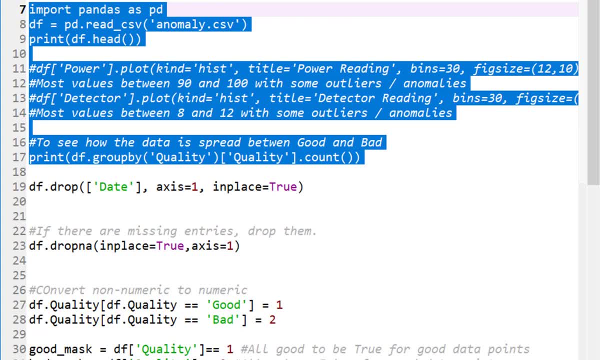 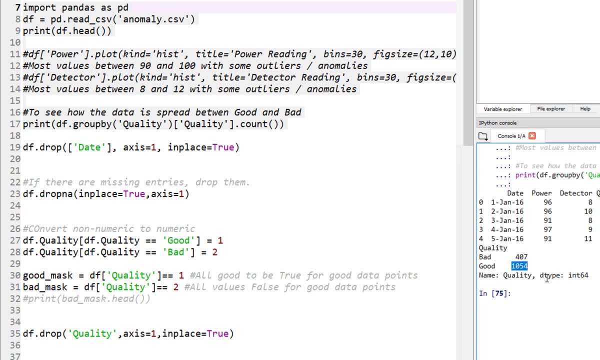 so you can actually look at. by the way, let's go ahead and run this up to this point. so now, here you can see, I have 407 bad data points and 1054 data. well, I say bad data points, data points that are labeled bad, and 1054 data points that are labeled good. okay, now, if you're doing classification, 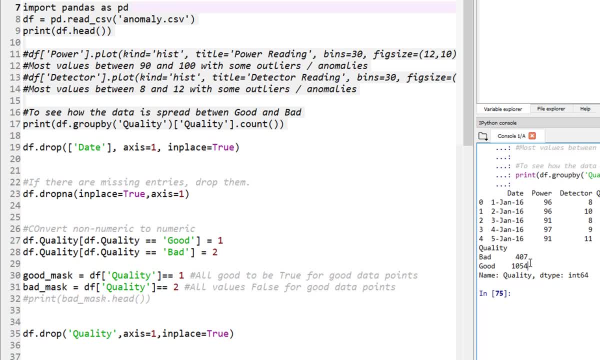 type of problem. right, okay, if you're trying to say: okay, if certain, as you know, create a model where you spit out good and also bad, then it's important to have like bad data points balanced with the good, maybe have like almost 1000 of each. then you can do some data augmentation or something. but 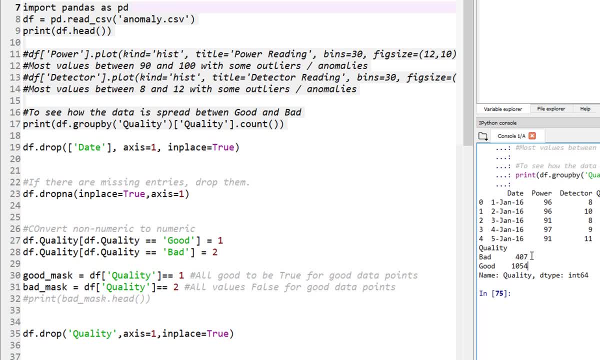 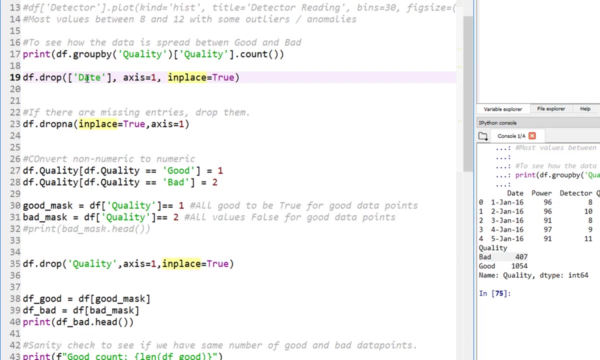 remember we are doing a anomaly detection, meaning we can work with 1054 good data points and completely ignore all the 1407 bad data points- well, ignore during the training process. but then we are going to use those data points to see how good our anomaly detection is working. okay, and here I'm actually dropping the date column right there. 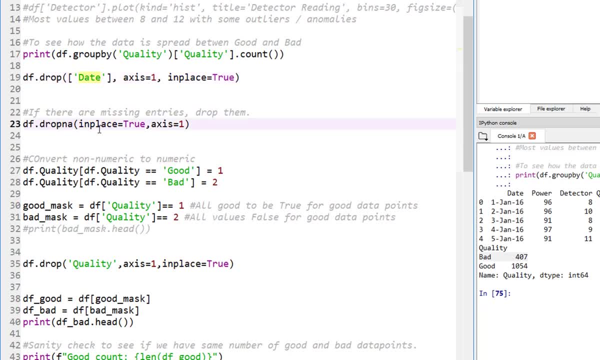 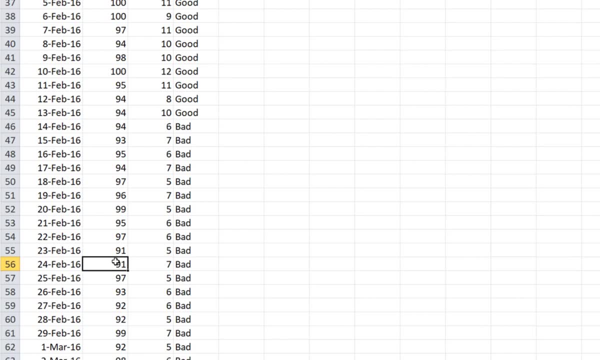 so that's what this line does, and here I'm dropping any missing entries. for example, here I have all values for every day, but sometimes, some days, you may not be taking the readings for power and detector. so if you have any blanks, one way to include those is by replacing the blanks with an. 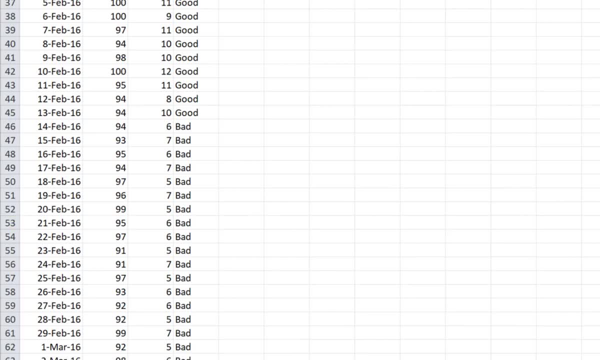 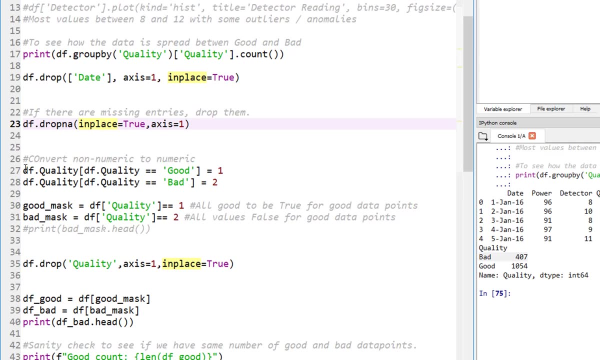 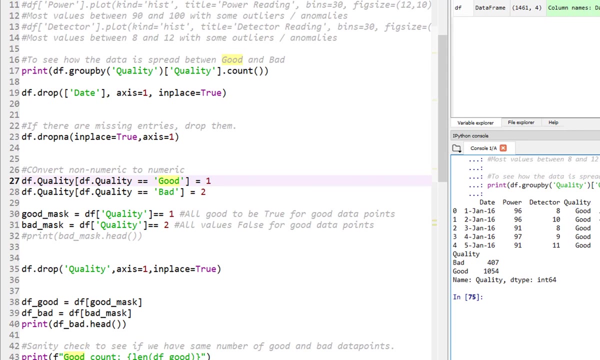 average of the value before and after. that kind of works. but if you have a lot of data points, go ahead and drop the the blanks. okay, that's what that line does over there and these two lines here. we are just assigning good equal to one and bad equals to two, so replacing the value good with a value of one. now we need to separate the good. 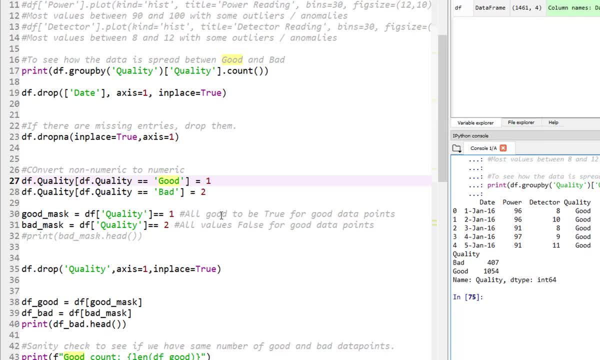 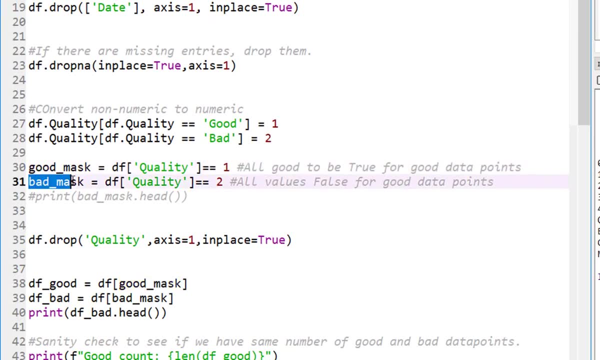 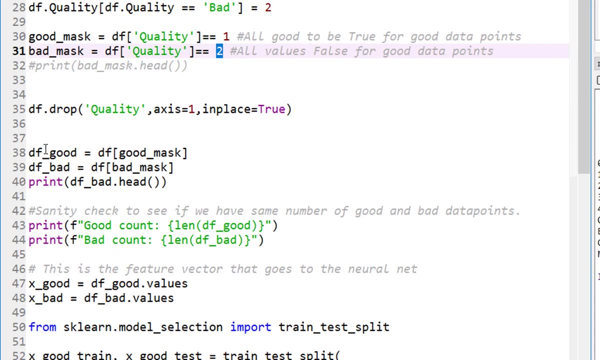 from the bad ones. so the way I chose to do that here is create a mask for all the data points where the value equals to one, and my bad mask is all the data points where my value equals to two. once I have that, then I can actually create a data. 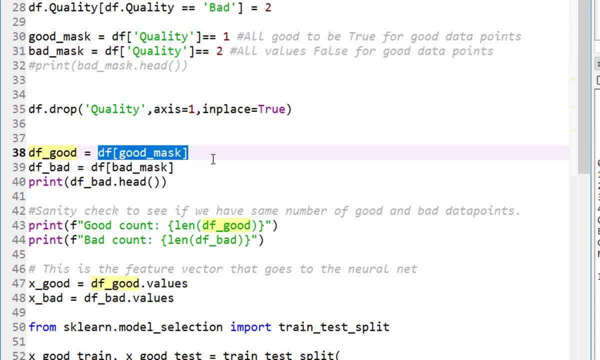 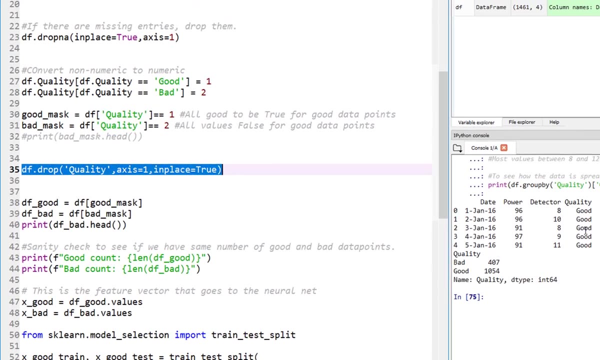 frame called a data frame good, with only the ones that are good, and data frame bad is the only the ones where the the label equals to true, you know, for bad data points. so that's what we're doing here, and also I dropped the quality column here. so we dropped this quality, uh, from our data frame. okay, 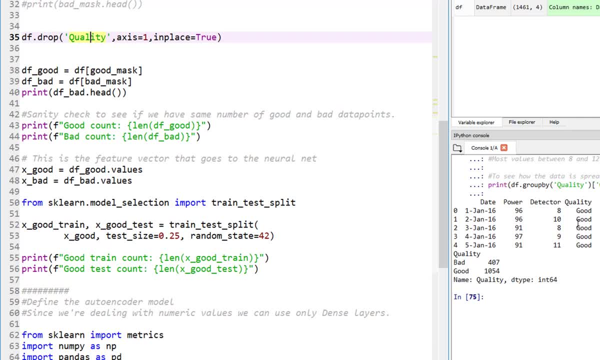 now, where do I go? uh, we drop the quality because, for training purposes, we only need power and detector values. right, we only need the values of real variables. we don't need the uh, we don't need the outcome as part of our training process. that's the reason why I dropped the quality over. 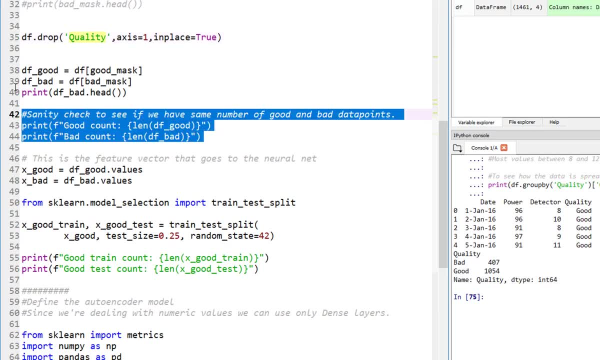 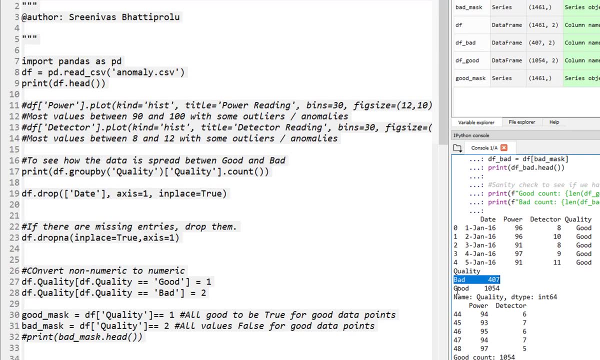 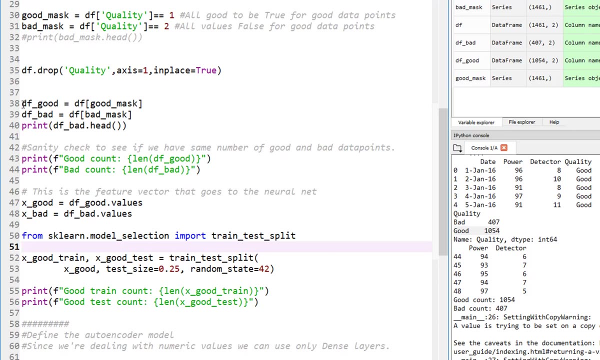 there. okay, so that's it. so, finally, if you, if I run the code all the way up to this point, you will see that, okay, we have initially 407 bad ones and 1054 good ones, and after separation and everything. so, if I go back here, what we are printing here is after: 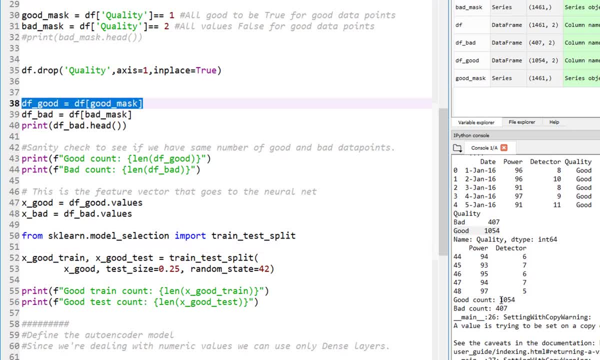 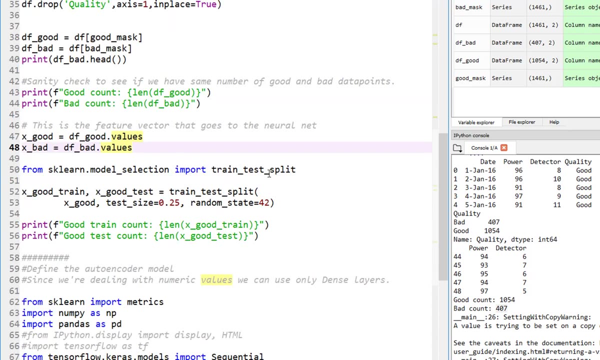 separating them as good data frame and bad data frame. I have 1054 good ones, 407 bad ones, meaning I didn't make a mistake. well, uh, uh, in this process, okay. so again a sanity check that I always try to do. okay, so what goes into our auto encoder is a vector, so the data frame itself is not good enough. 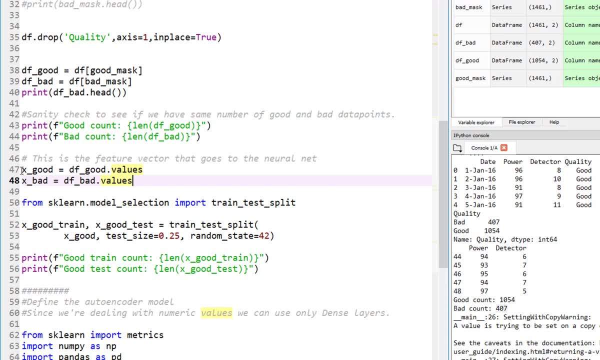 so I'm going to extract the values from my data frame and assign it to a vector right there. okay, so these are the feature vectors that I'm going to use. in fact, the good is the only feature vector I'm going to use as part of my 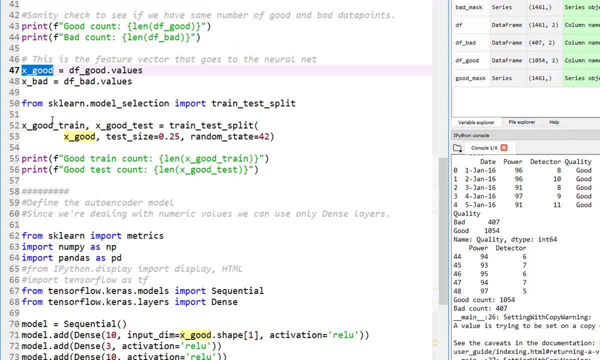 neural network. okay, so now, instead of using all the data points in good meaning, all the 1054 data points- I want to hold out 25 percent as validation data or testing data. so the way I do that is using the train test split method inside this library, scikit-learn model selection. 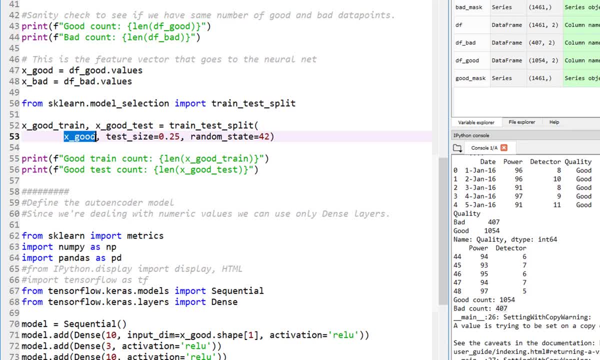 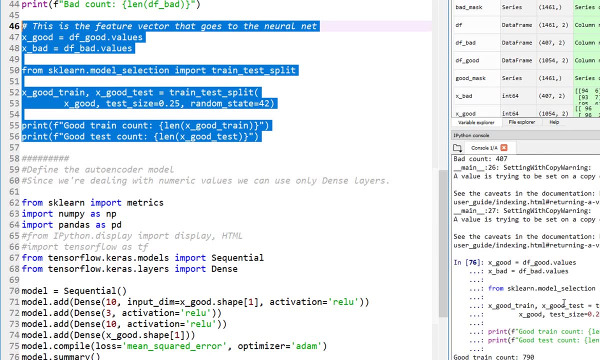 so 75 percent of my good data is assigned as x- good train. 25 is assigned as x- good test. okay, that's all it is. now, again, you can go ahead and print this to see how much good, how much bad. so let's run this. so, as you can see, of all the 1054 data points, 790 are going to be used as part of my. 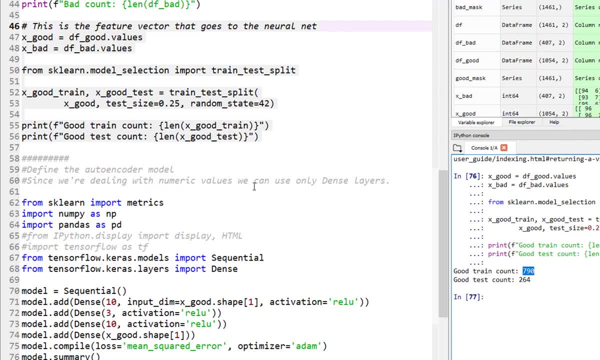 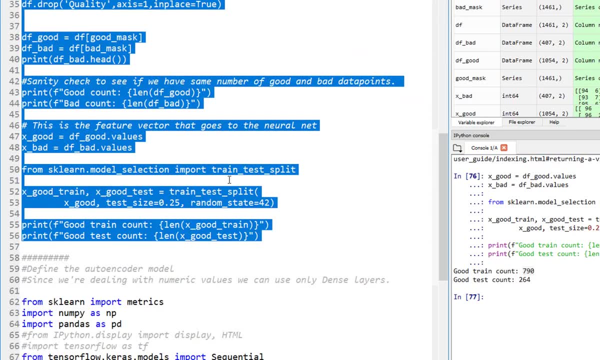 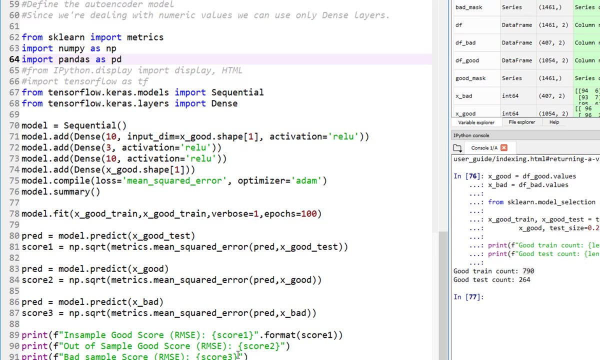 training, and 264 are going to be held out for testing or validation purposes. so this is how I I kind of designed my data, and I already explained this part right. so, uh, let's go ahead and run it. so eventually, we are going to look at what the score is for my uh, for. 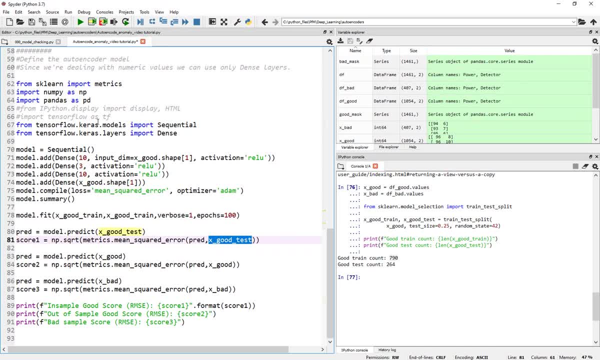 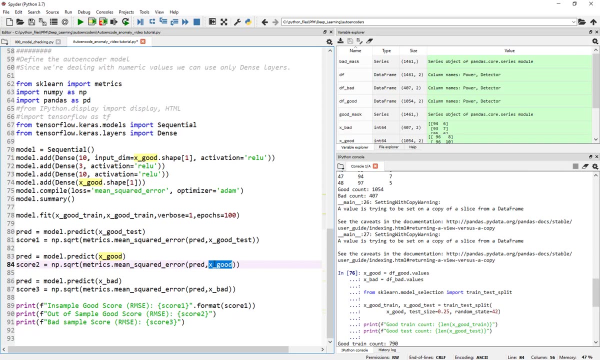 my prediction on good test data set. this is the 25 data set that we are holding out. how it is for my x good, which is the entire data that we used for well, that we uh have for good data points, meaning 1000, whatever 54 data points- and then how well the prediction is. 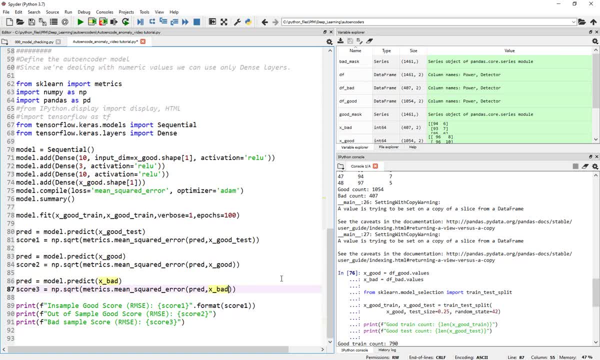 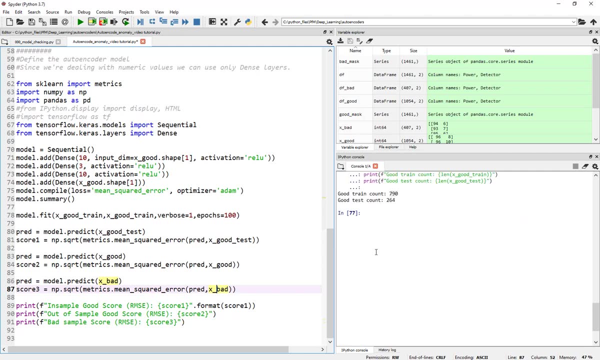 going to be on the bad data points and again, the assumption is- because this is anomaly detection- the good- these two probably are very close- and the bad ones, uh should be probably at least 50 percent uh higher, or you know uh error. so let's go ahead and run this. where are we? okay, let's run. 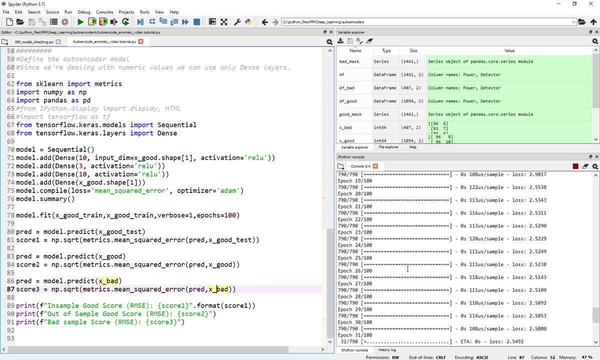 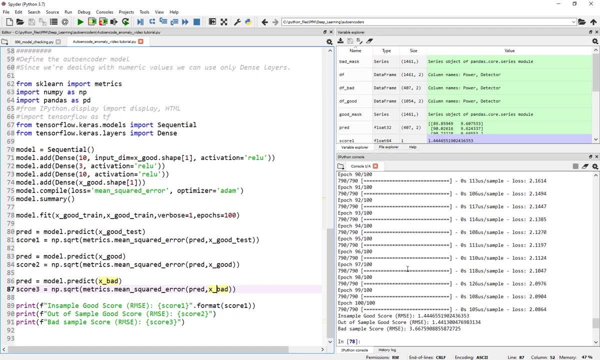 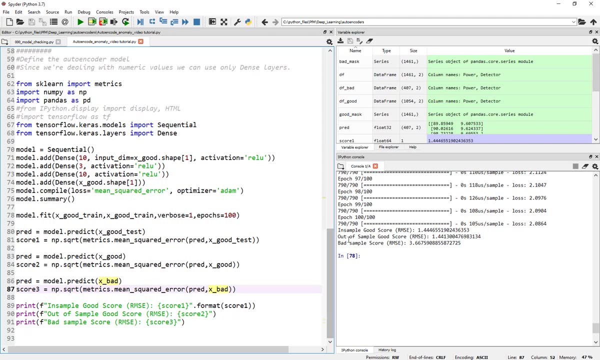 this for 100 Epochs, I believe. there you go, okay, finally, here are the values. so, uh, I should have said out of sample. this is not out of sample. this is basically the entire data set. but anyway, the the, the good score, seems to be centered around.